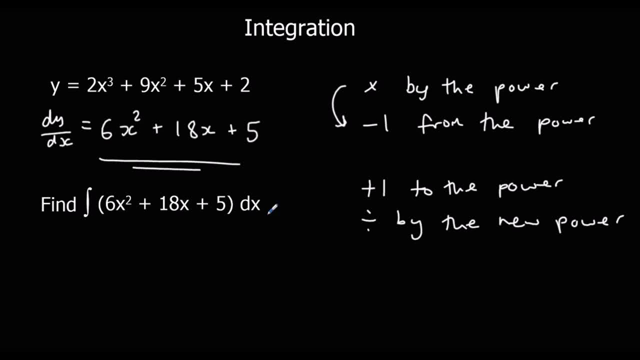 So that's what we've got here, what we got by differentiating with respect to x. So the process plus one to the power, add one to the power. So we're going to add one to the power and then divide by the new power. 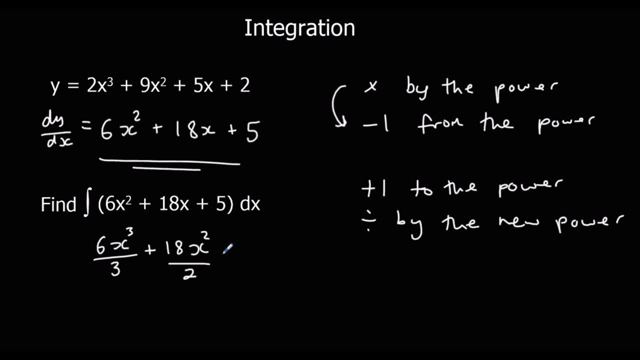 So add one to the power, divide by the new power. We've got five x zero here. So if I add one to the power it'll go to five x, And then you see we had a two here that disappeared. So whenever you differentiate, if it's just a number it's going to disappear. 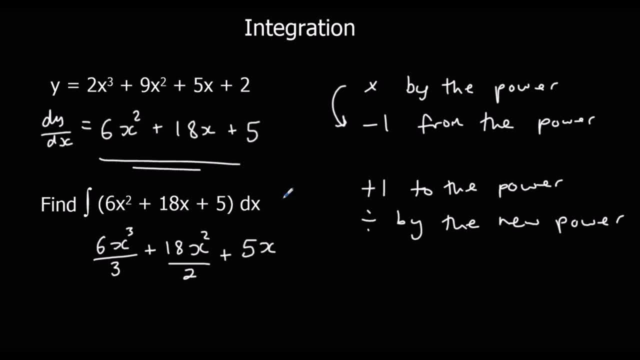 So in order for integration to undo that, what we do is we write plus c on the end. So it's kind of like a third step for integration: Add one to the power, divide by the new power and plus a c on the end. 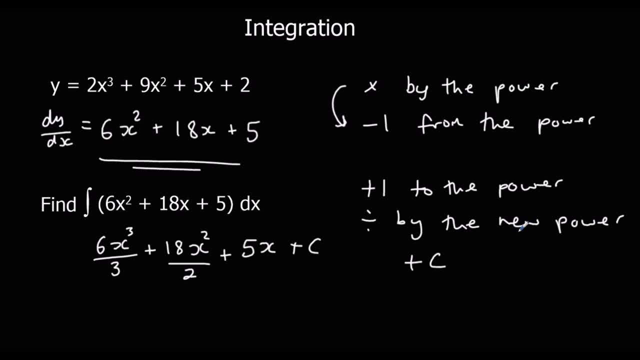 So that c just represents any number that could have been there originally. that would have disappeared when you differentiated it. So whenever you integrate, just remember plus c. We can simplify this. So six over three is two, 18 over two is nine. 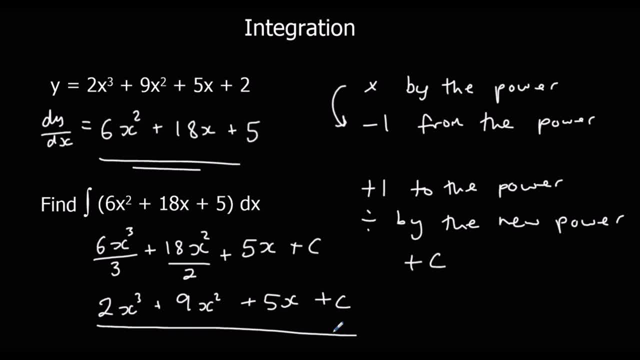 And then plus five x plus c. So that is how we integrate. Now we've got no way of knowing what the c was here. Well, we do know it was two, But if this was just the question, if that was the whole question, 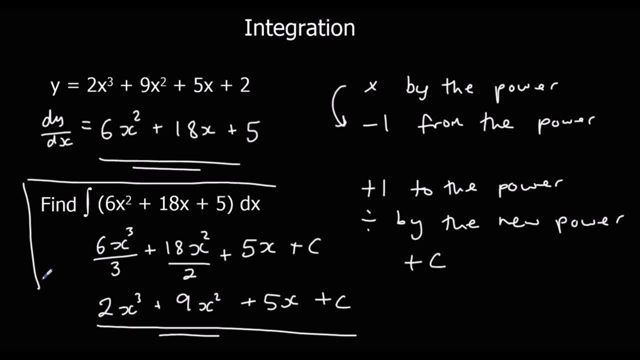 we would have no way of knowing what the c was, So we just leave it as plus c, unless we're given the information in order to find out what it is. So in this case, just plus c on the end, and that's absolutely fine. 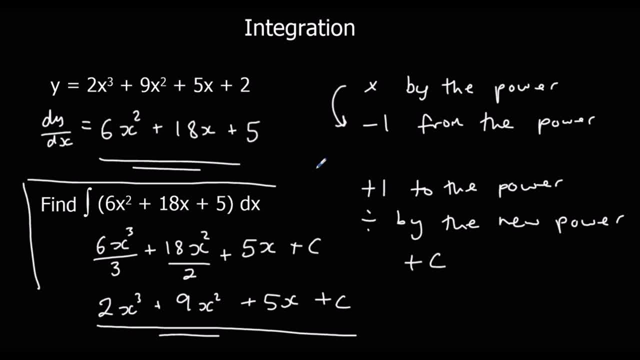 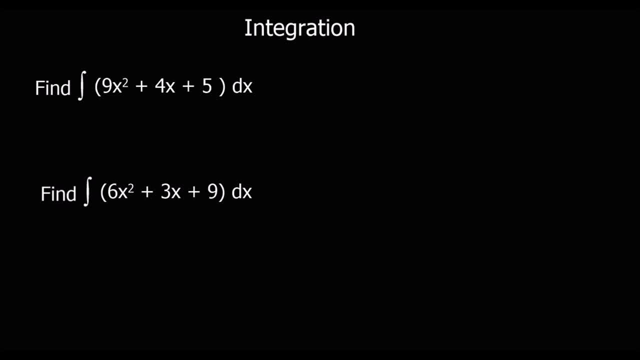 So integration, we're going to have plus one to the power, divide by the new power And then plus c on the end. Okay, let's have a look at doing some questions. So we're going to follow the process: Add one to the power, divide by the new power and plus c on the end. 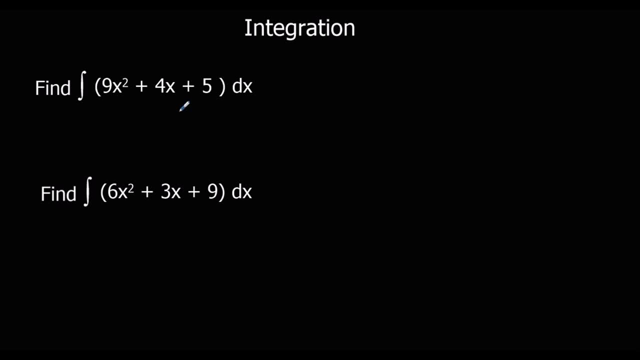 So find the integral of this. with respect to x, That just means we're integrating x's, So we're going to add one to the power. divide by the new power, Add one to the power, So it'll be one that goes to two. 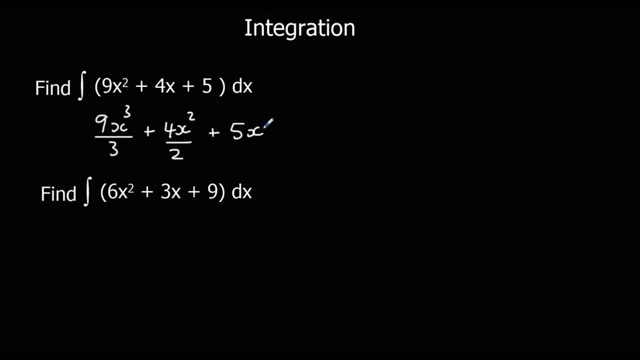 Divide by the new power. Add one to the power. We don't need to divide by one, because five divided by one is just five And plus c on the end. We can simplify these Nine divided by three. Can I squeeze the answer in? 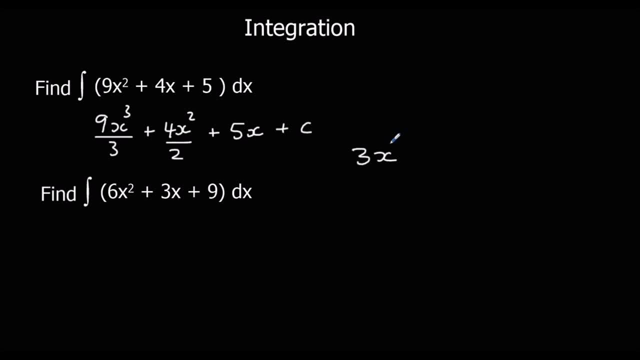 I'll do it over here: Nine divided by three is three, So we've got three x cubed. Four divided by two is two, That's two x squared plus five x plus c. That's the answer. So same again. 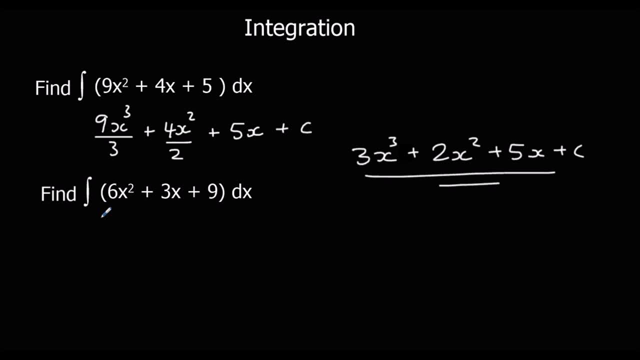 Same again. Follow the same process. Add one to the power divide by the new power and put a plus c on the end. So let's add one to the power divide by the new power. Add one to the power divide by the new power. 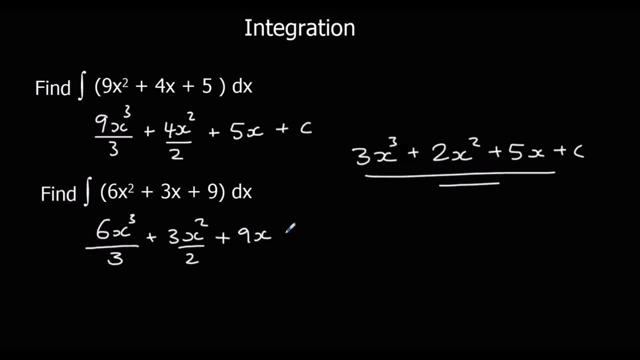 Add one to the power divide by one again. We don't have to write that Plus c. We can simplify six over three, which is two. Three over two. we can leave as three over two. Okay, X squared plus nine, x plus c. 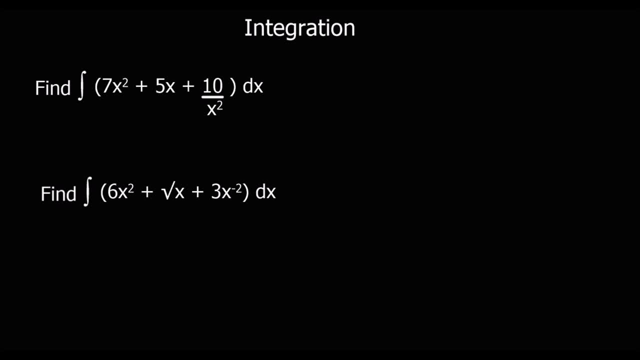 Okay, These ones are a little bit trickier because we've got to do some rearranging, some simplifying before we can integrate them. So in this case we've got ten over x squared, So we can't integrate ten over x squared. 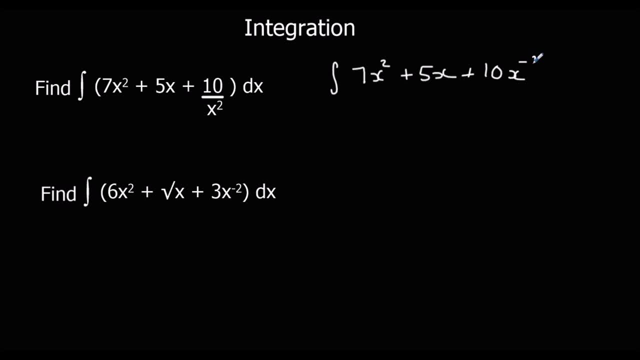 But if we change that, Change it to ten x minus two, So ten over x squared is the same as ten x minus two- Then we can. So what we're going to do? simplify it. first We've done that, Then we're going to follow the same process. 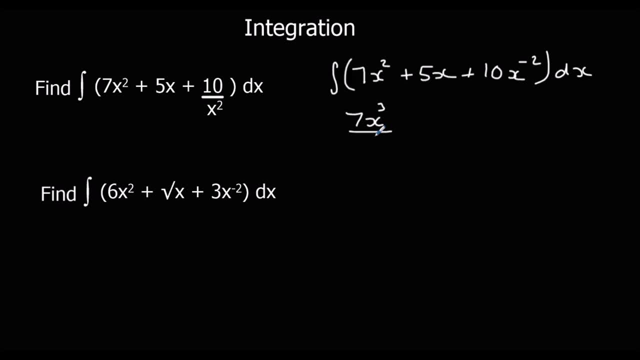 So we're going to add one to the power and divide by the new power. Add one to the power, divide by the new power, Add one to the power, divide by the new power, And plus c, Plus c on the end. 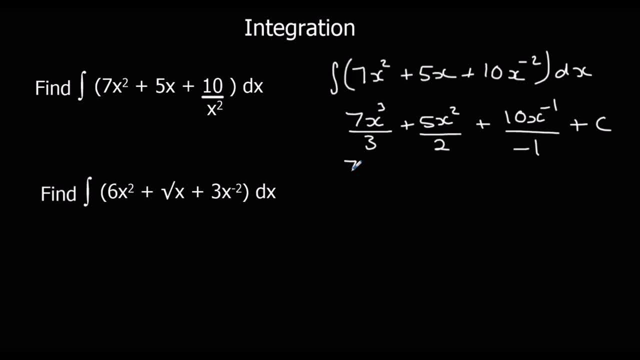 Now we're going to simplify this: Seven over three is just seven over three. Five over two is just five over two. Ten divided by minus one is just minus ten, And a positive divided by a negative is a negative Plus c, And that's our final answer. 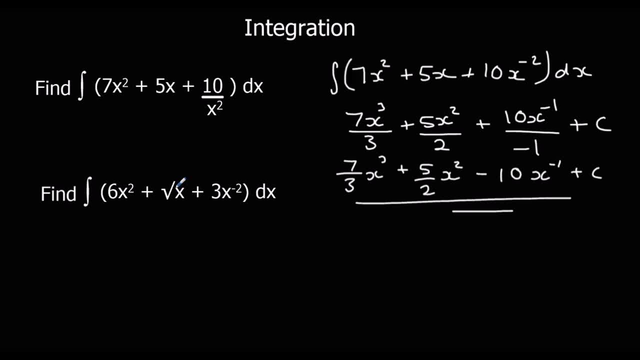 Okay, Same again. here We can't have root x, but we can change it to x half, So six x squared plus x half, plus three x to the power of minus two. And again we're just going to follow the same process. 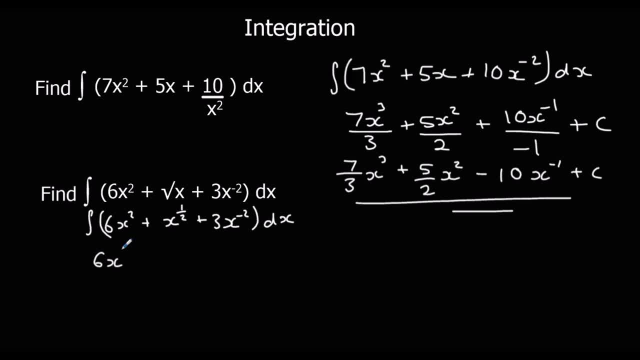 So we're going to add one to the power and divide by the new power. So two plus one is three. Divide by three, A half plus one is one and a half, So three over two. And we're going to divide by three over two. 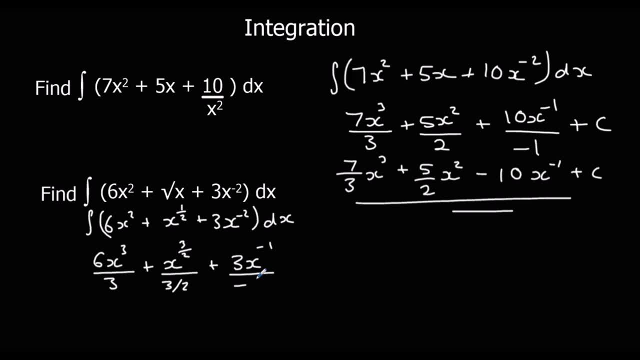 And then minus two plus one Is minus one. Divide by minus one And plus c, Don't forget the plus c. So six over three is two. So we've got two x cubed, So we've got one x here. 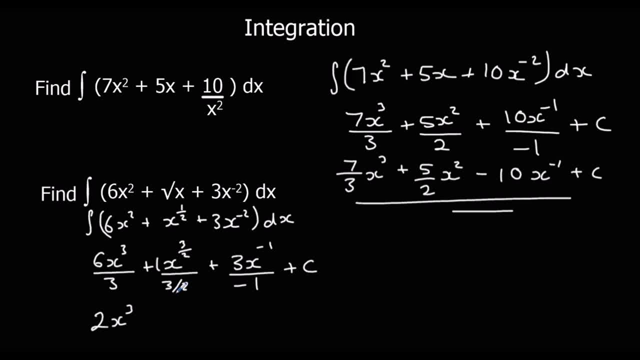 One divided by three over two. When you divide by a fraction, just flip it and change it to a time. So dividing by three over two is the same as times in by two over three. So one times two over three is just two over three. 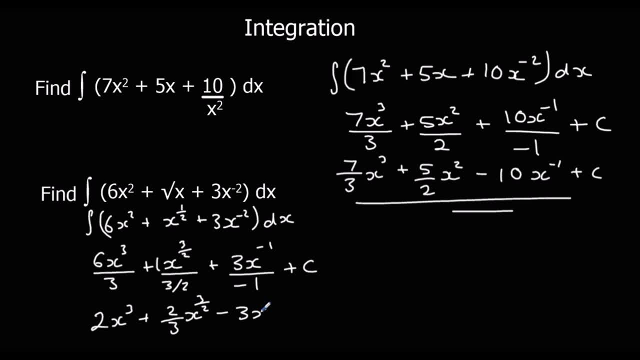 X to the power of three over two Minus three. x to the power of minus one. Positive divided by negative is a negative Plus c, And that's our answer. Okay, here's another few. Pause the video. give them a go. 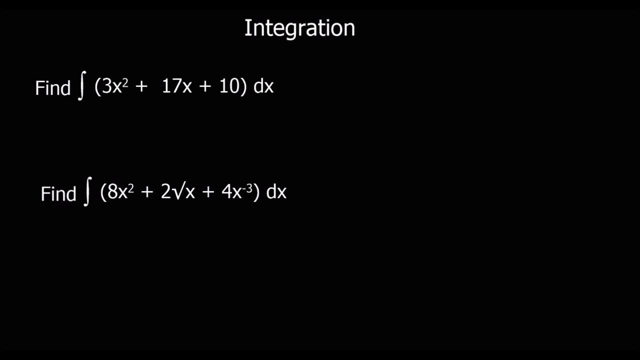 Okay, so integrating, So we're adding one to the power, Dividing by the new power And plussing c on the end. So we're going to add one to the power. So two plus one is three, Divide by three. 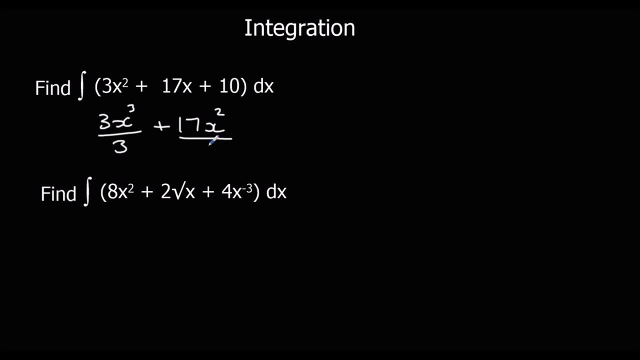 We've got x one here, So that goes to x. squared Divide by two Ten goes to ten x, And we plus c Three over three is well, they cancel. So we've just got x cubed, All right, the side here. 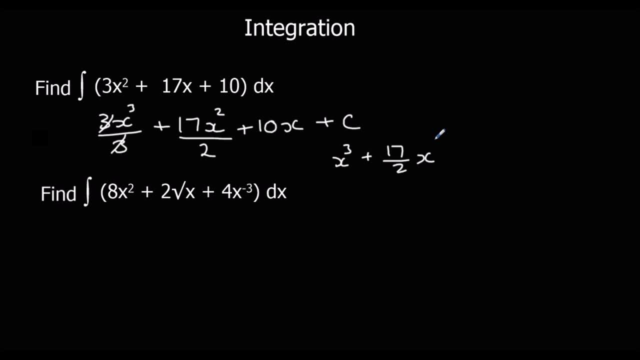 X cubed plus seventeen over two x squared Plus ten x plus c. Okay, the second one. We have to change the Root x to x half before we can integrate it. So we've got eight x squared Plus two x half. 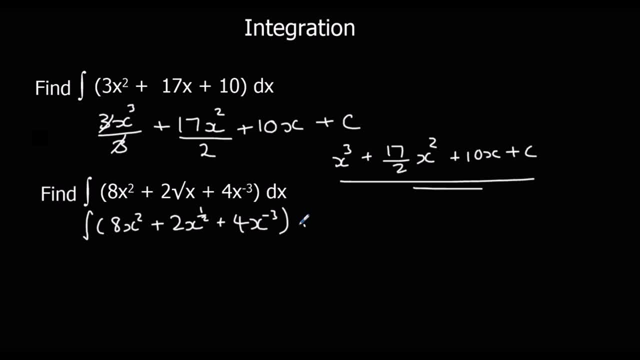 Plus four x to the power of minus three. Again the same process. Add one to the power, Divide by the new power And plussing c on the end. So two plus one is three. Divide by three, Half plus one is three over two. 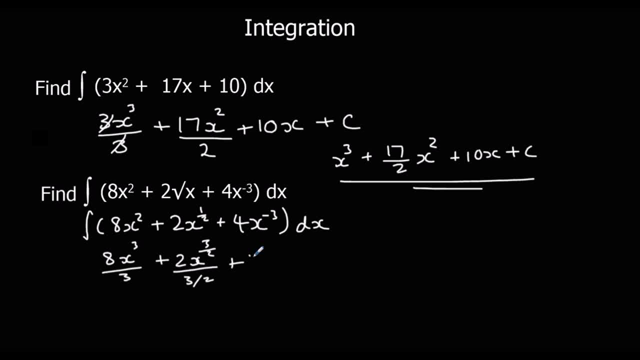 Divide by three, Three over two, Minus three plus one is minus two, And we're going to divide by minus two And plus c on the end. So eight over three, Eight over three, x cubed, We've got two divided by three over two. 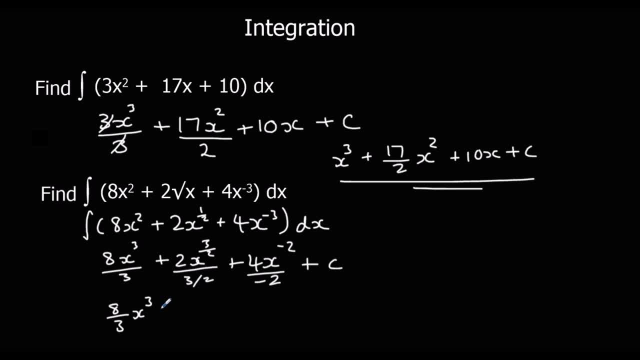 It's the same as two times two over three, So two times two over three, Two times two over three. Think of it as two over one times two over three, Which is four over three. So four over three. x to the power of three over two. 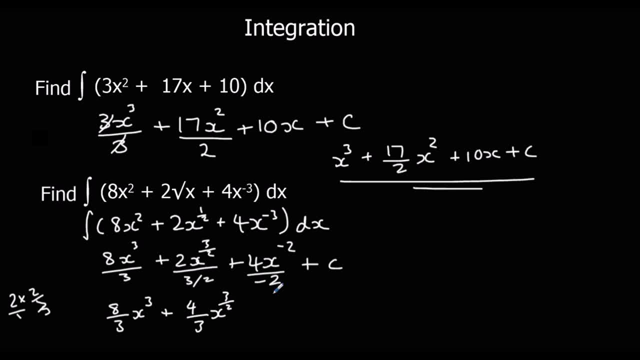 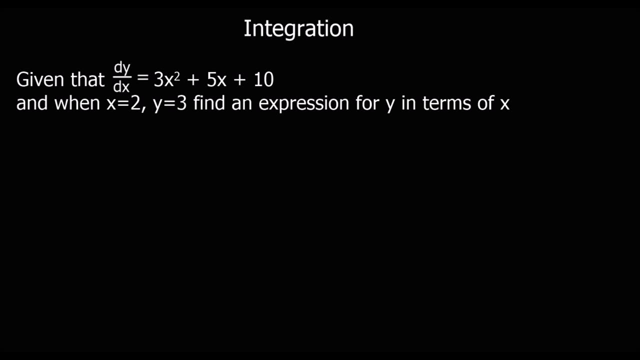 Four divided by two is two Positive. divided by negative is a negative. So negative: two x to the power of minus two Plus c. Okay, here we've got another integration question. It says: given that dy dx is equal to three x squared, 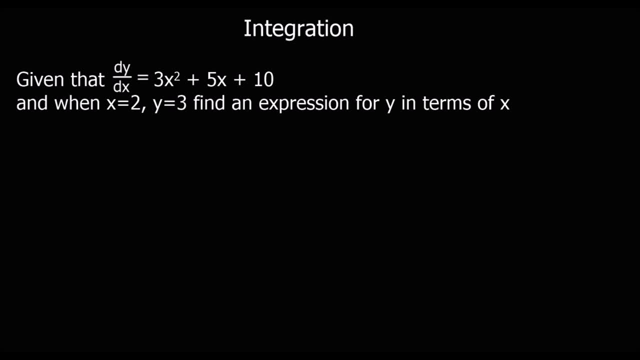 Plus five, x plus ten, And when x is two, Y is three, Finds an expression for y in terms of x. So what they're asking us to do Is to go from dy, dx Back to y. So that means undoing differentiation. 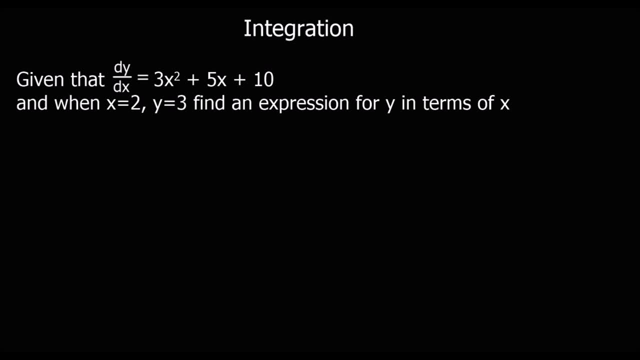 And the undoing of differentiation Is called integration. So they've given us X is two and y is three. That means this time we can work out what c is. So when we, After we integrate, We're going to substitute. 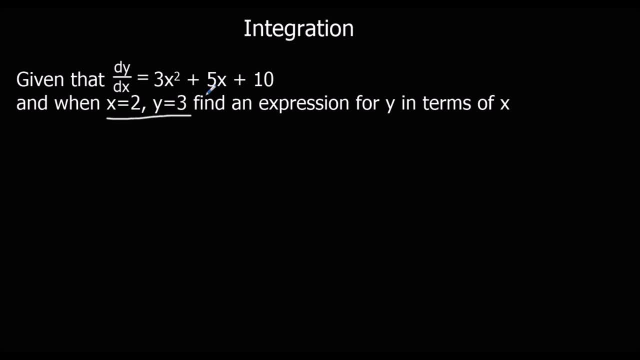 The two and three in To find c. So the first thing we have to do here Is we need to integrate it. So Dy dx, when we integrate, Is going to go to y, And then we're going to integrate each of these terms. 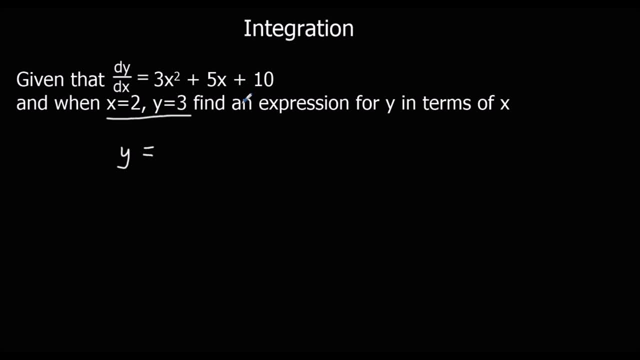 So that means adding one to the power And dividing by the new power. So we've got three x squared first. So we're going to add one to the power And divide by the new power. It's five x one at the moment. 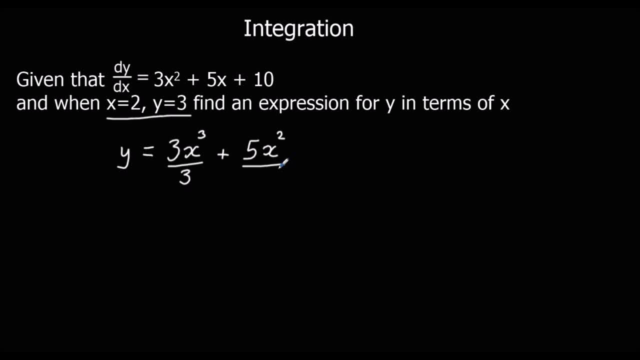 So when we add one to the power, I get five x squared And it's ten x Zero at the moment. So that'll go to ten x to the power of one. Divide by one. I'll put the divide by one. 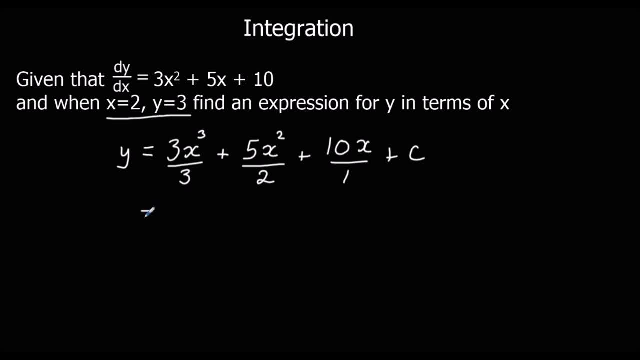 And plus c. So just simplifying these terms, That'll give me X cubed Plus five over two, x squared Plus ten, x Plus c. So I've integrated it And now I'm going to substitute in My two and three: 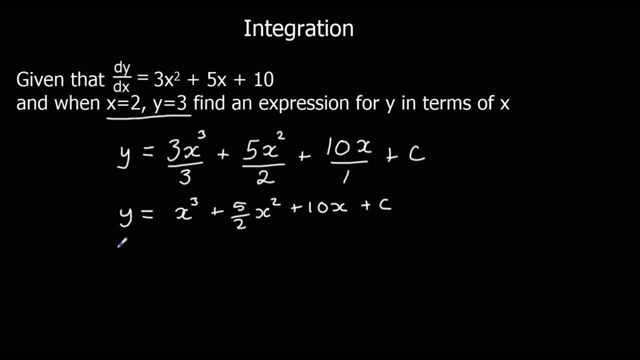 To find out what c is. So I'm going to substitute three In for y And two In for all of the X's. So I'm just putting brackets And substituting the two in, So we've got three. 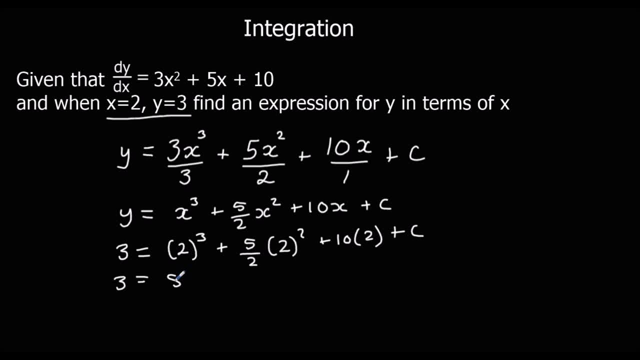 Equals: two cubed Two times two times two Is eight. We've got Five over two Times by Four. Five times four Is twenty over two, Which gives me ten, And ten times two Is twenty Plus c. 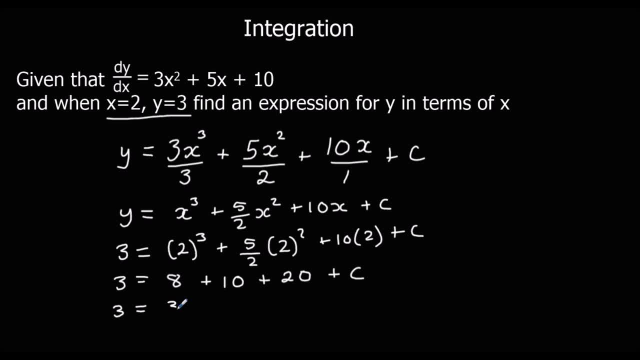 So that gives me three equals Thirty eight Plus c. Take away thirty eight from both sides, So I've got minus Minus thirty five Is c. So the expression for y in terms of x Is: y equals X cubed. 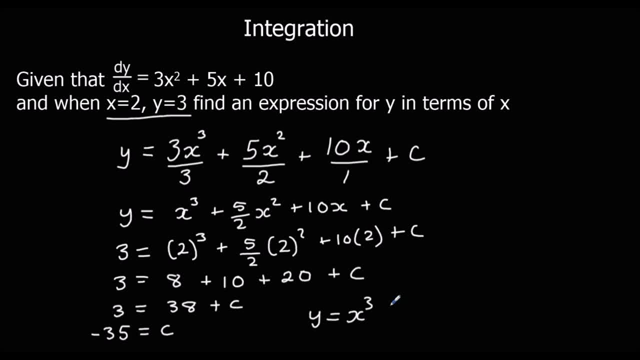 So I'm taking it from this line And just substituting my c in Plus five over two X squared Plus ten x Minus thirty five, And that is my answer. Subtitles by the Amaraorg community. Subtitles by the Amaraorg community. 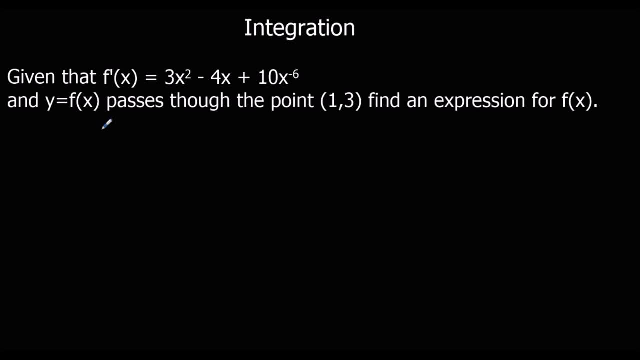 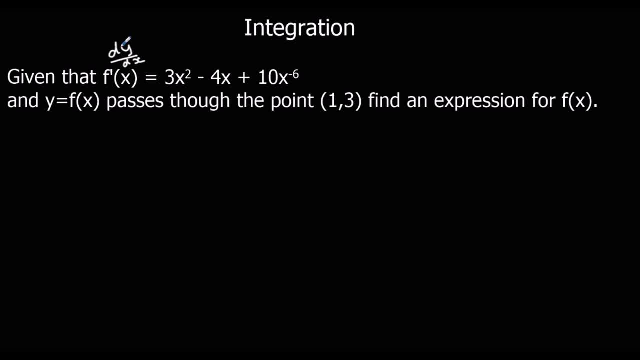 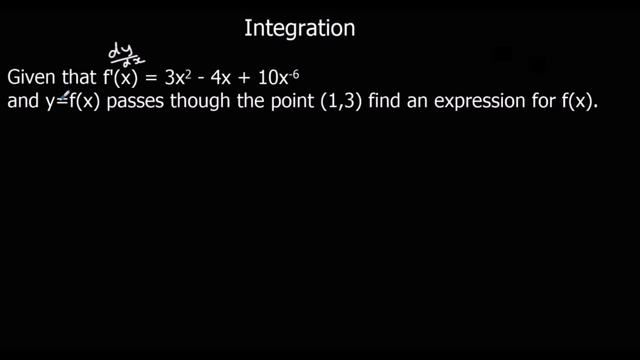 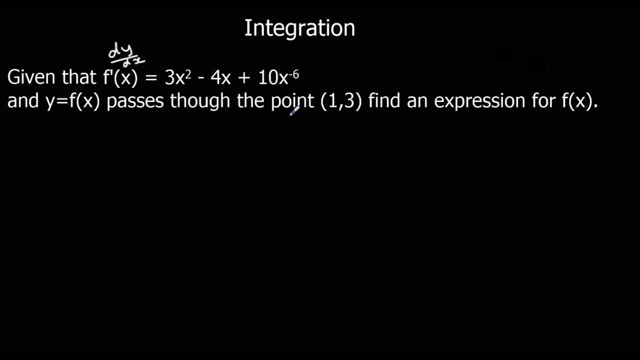 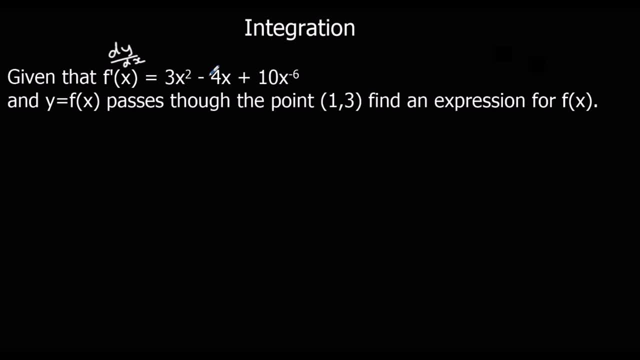 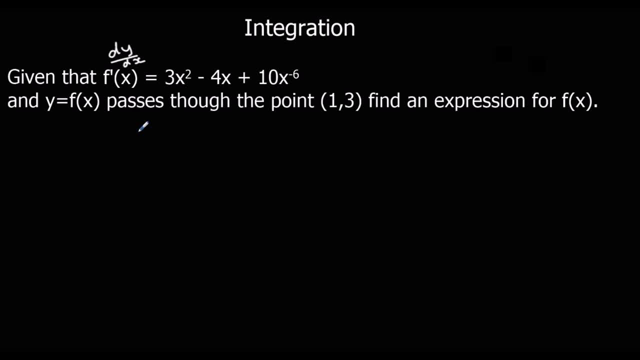 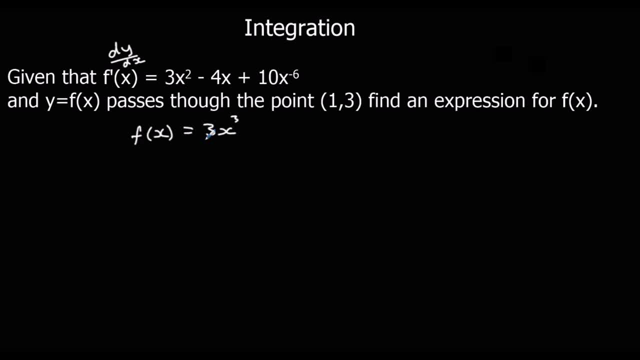 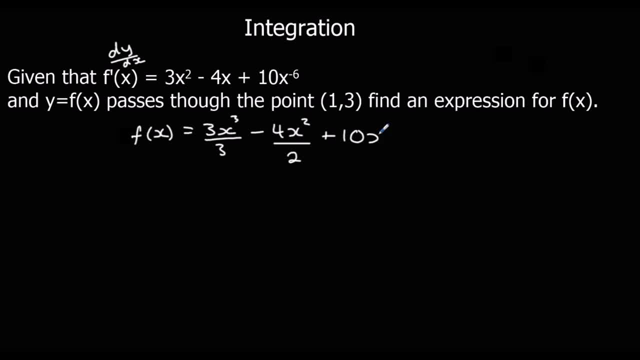 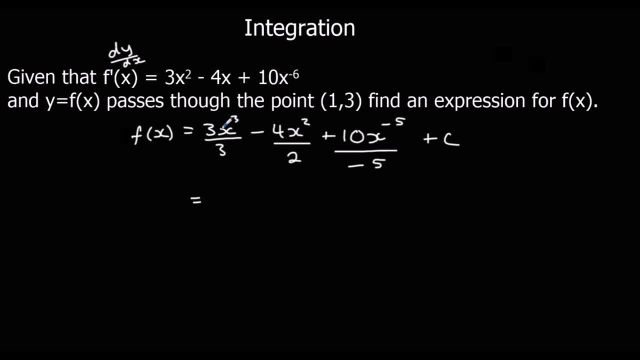 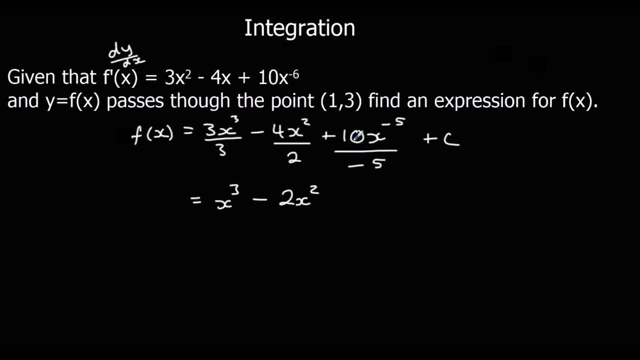 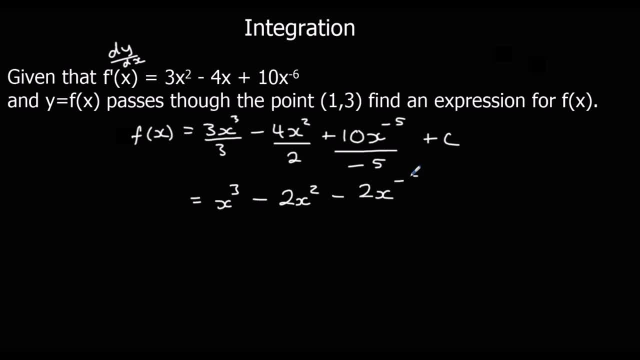 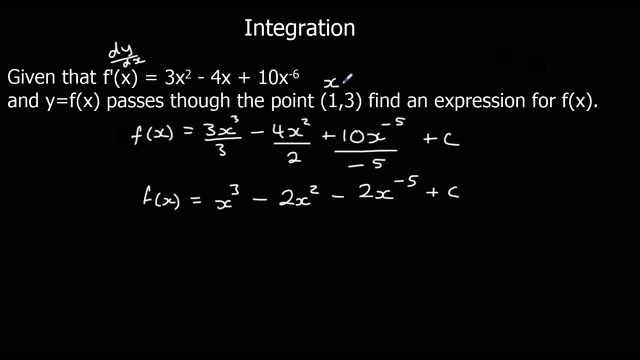 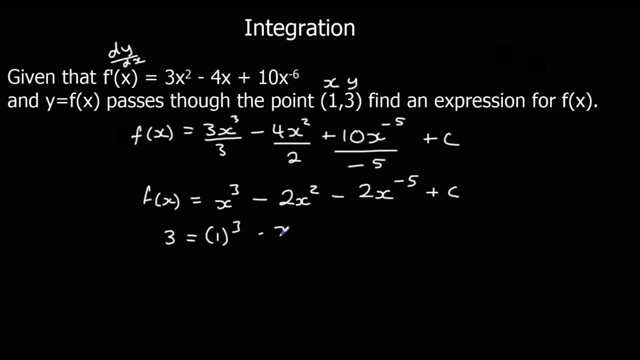 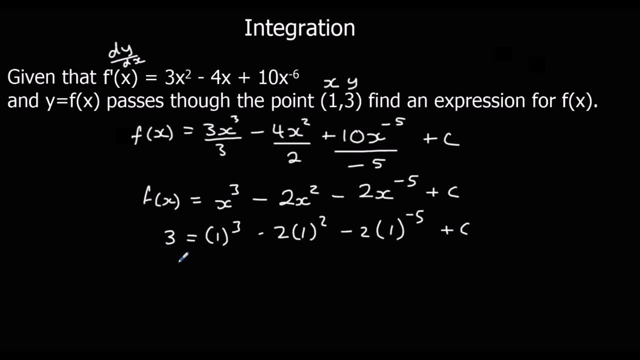